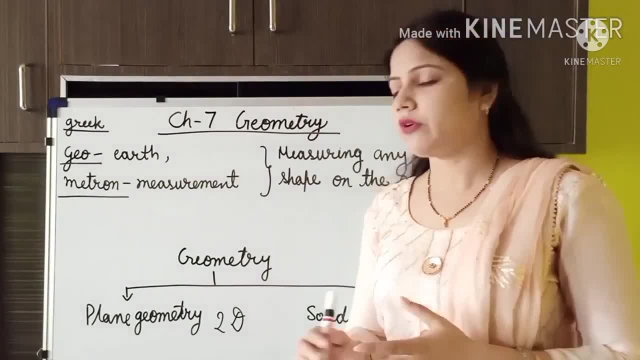 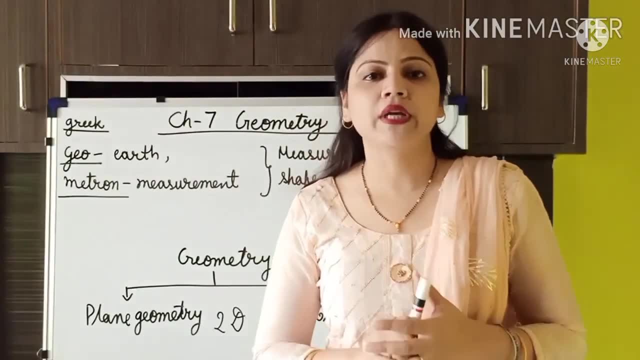 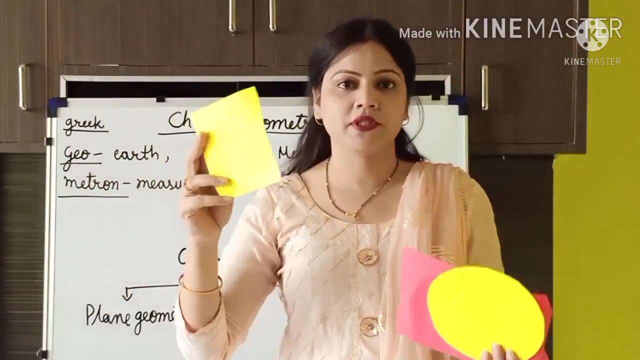 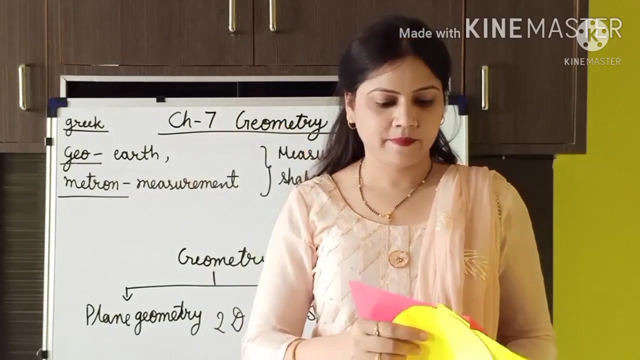 Solid geometry. But before starting the solid geometry, we will just revise the plain geometry. Okay, Plain geometry means the shapes that are two dimensional. Two dimensional means what? As you can see, I have some shapes. Which shape is this? Very good Square, This one Circle, This is rectangle. Yes, 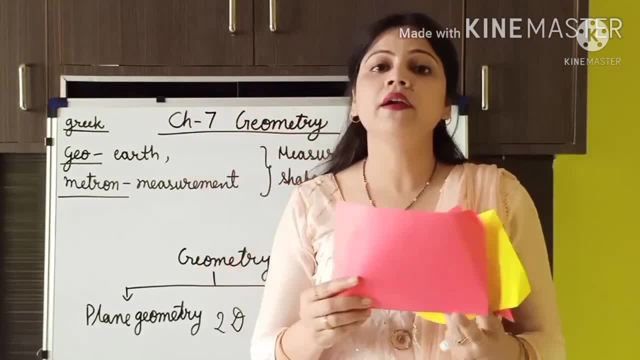 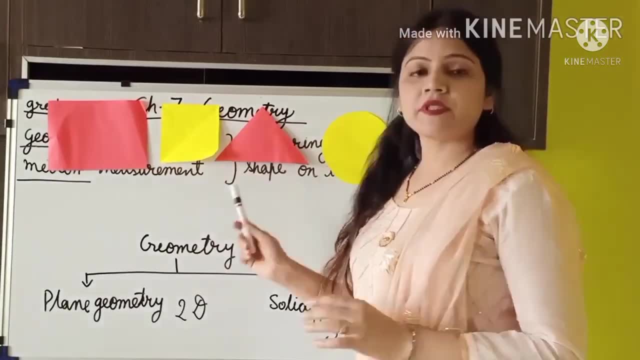 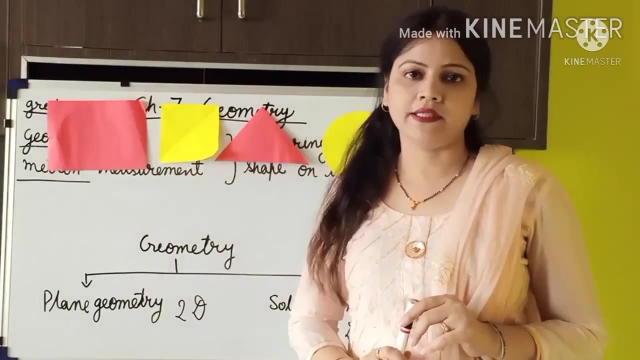 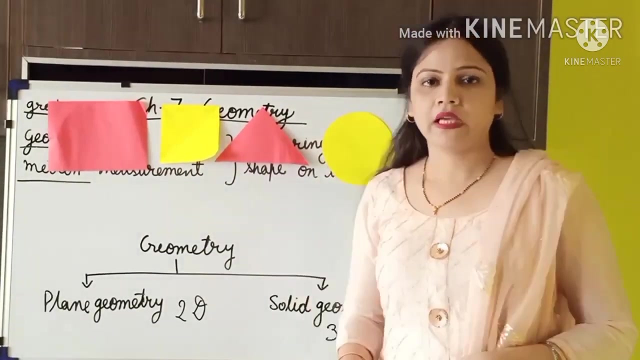 This is triangle, So these shapes are two dimensional shapes. First let me paste these shapes here. So these shapes are 2D shapes, Means it has only two dimension: The length and breadth, Okay, And these shapes we can easily draw on a sheet of a paper. Solid geometry is three dimensional in shape. Three dimensional means what? 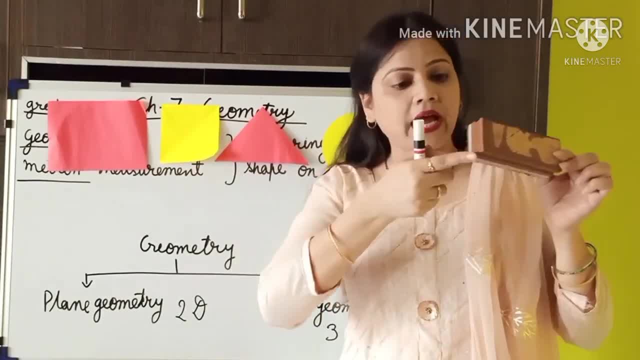 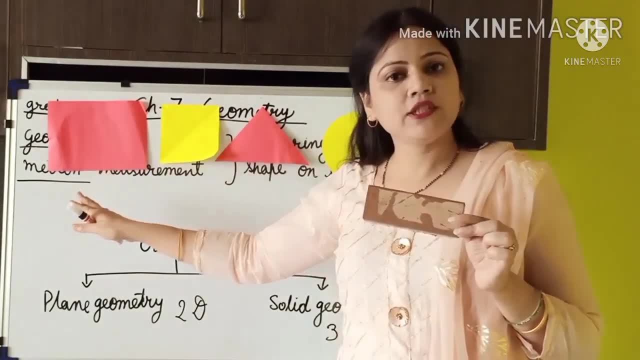 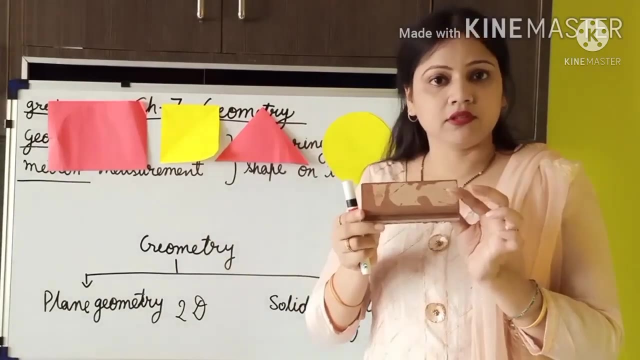 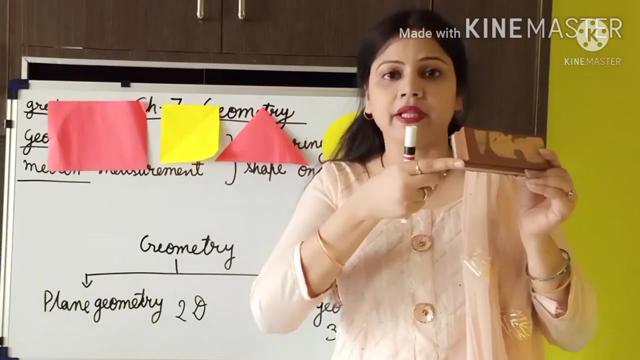 It has the length, the height and also the breadth. Okay, Not like the plain figures. The plain figure we can easily draw on a sheet of papers. It has only two dimension, Okay, Breadth and length. But the solid shapes are of three dimension. It has also the length, height and breadth. These are called the solid figures. Okay, Okay, So in this class you have to learn about the solid figures. Okay, So in solid figures we will learn about three different types of surfaces. Okay, What is surface? The top of anything is called the surface. Like, if you have a dining table in your home, then the top of the dining table is the surface of that. Okay, So in the solid shapes we will learn about three different types of surfaces. The first one is plain surface. What is plain surface? 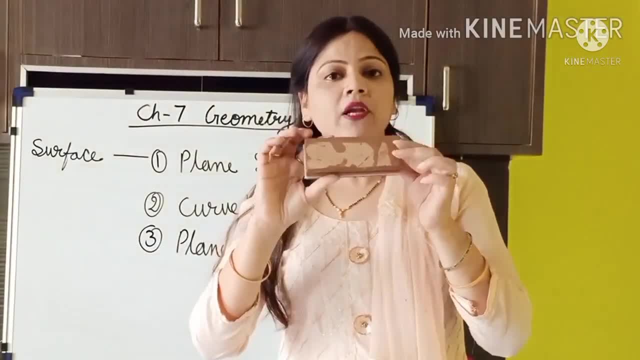 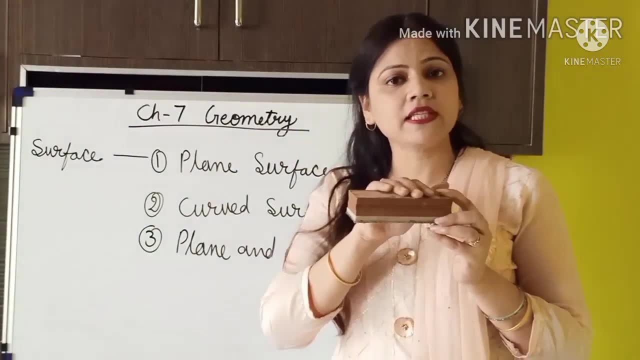 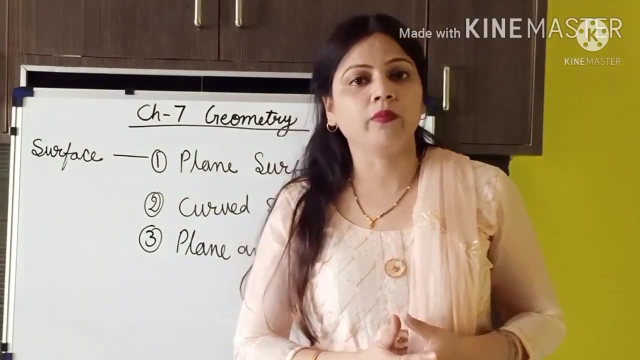 surface, like I have shown here. This is the example of cubite. Okay, So the top of the cubite is plain. Okay, So the surface of this cubite is plain. Similarly, like that, you can also see the floor of your home. This is also plain. The surface is plain. Okay, Now the 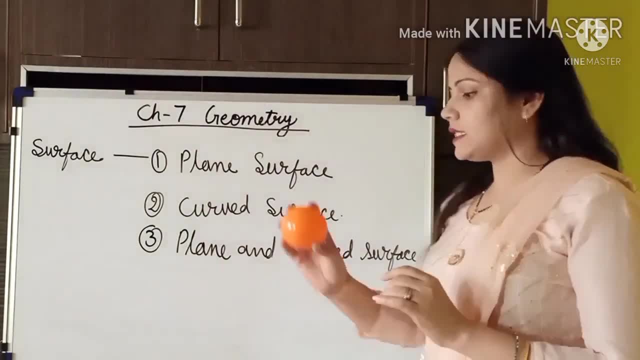 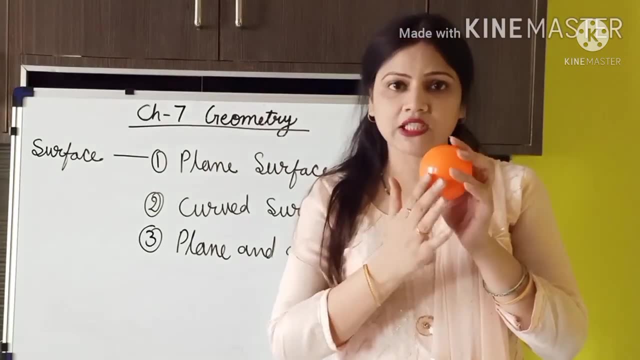 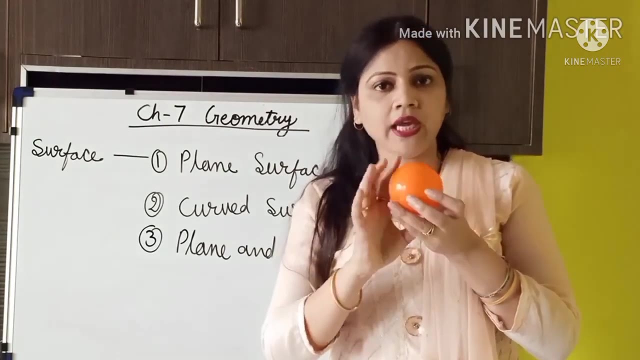 another kind of surface is curved surface. As you can see here I have a ball, So this ball is curved in surface. If you will touch it, it is not plain in any manner. Wherever you will touch it is curved. Okay, So the ball, the orange, the globes, these are the 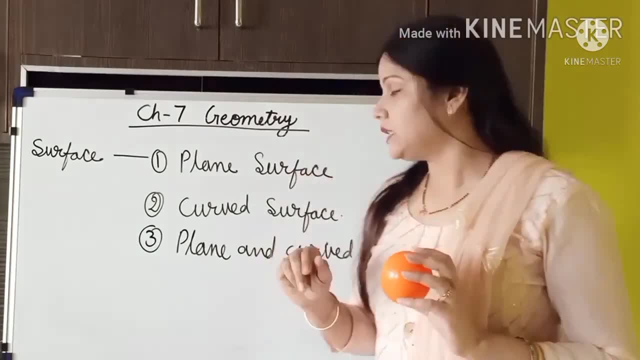 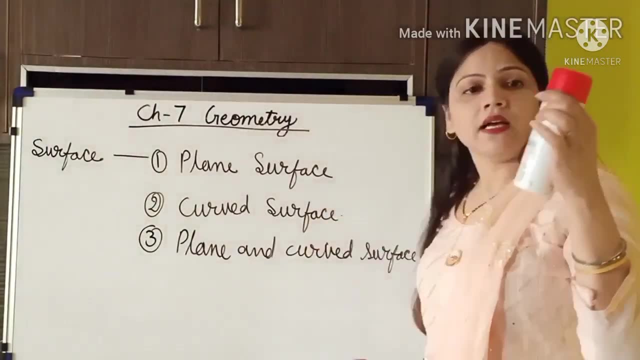 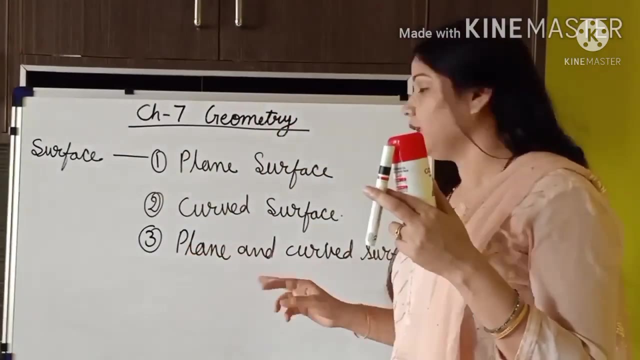 examples of curved shapes. Now, the third type of shape surface is plain and curved surface. Like you can see this: This is a powder and this is a marker. Okay, Both of these are the examples of plain and curved surface. How You can see this. 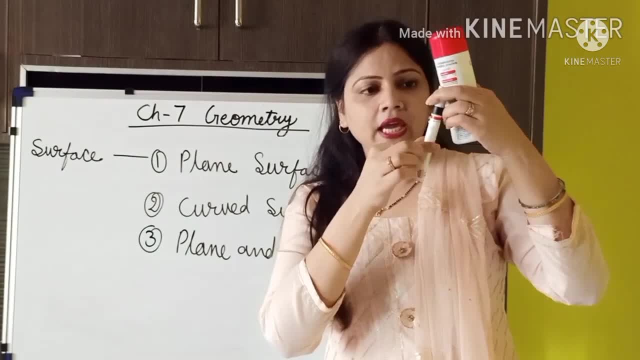 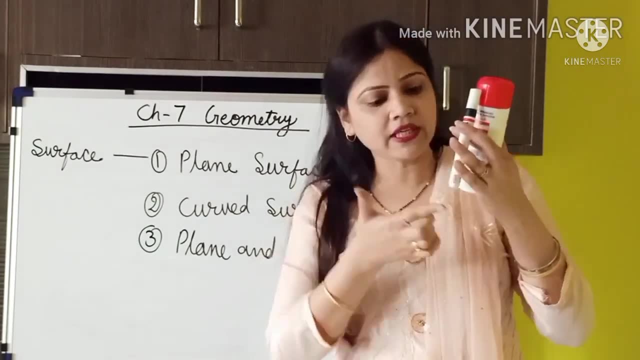 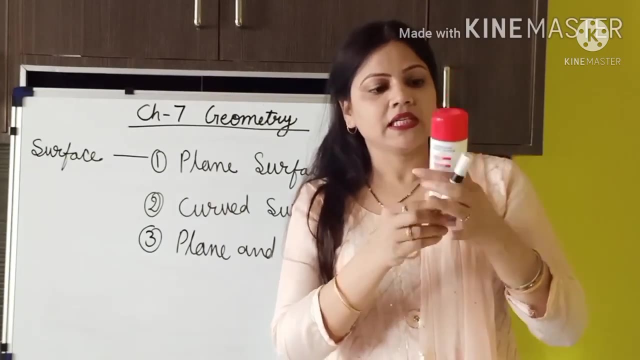 one. This side is curved in shape- Okay, But the top and bottom is flat in shape, Okay. So this is flat surface. The top and bottom is flat in surface, while this area is curved surface, Similarly like this also, This is in the middle. This is curved surface, and 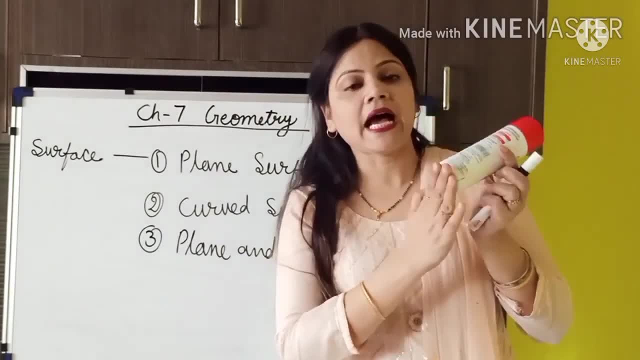 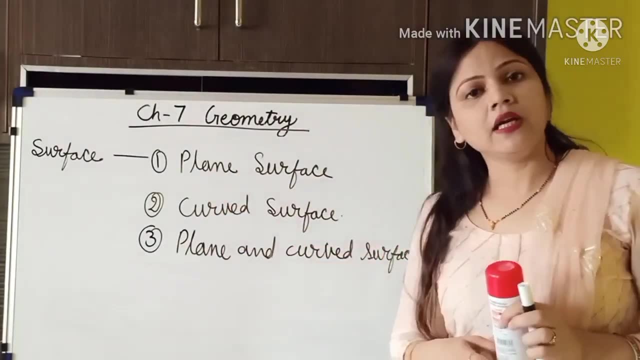 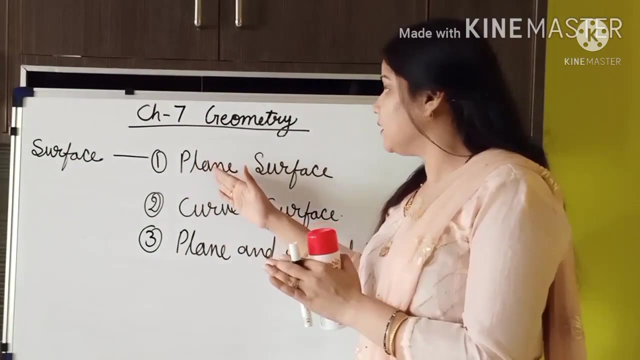 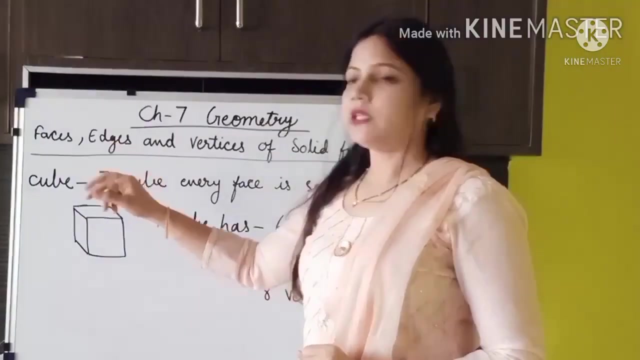 in top and bottom it has plain surface. Okay, So these three are clear: The plain surface, curved surface and plain and curved surface. So all the three dimensional shapes, all the solid shapes, have either plain, curved or plain and curved surfaces. Okay, Now we will. 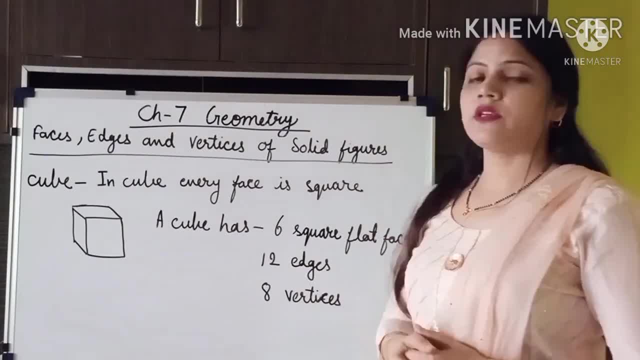 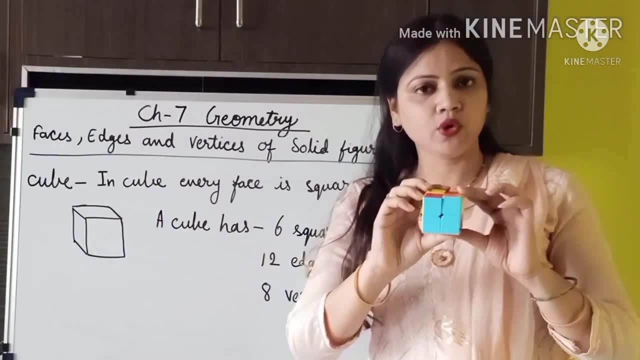 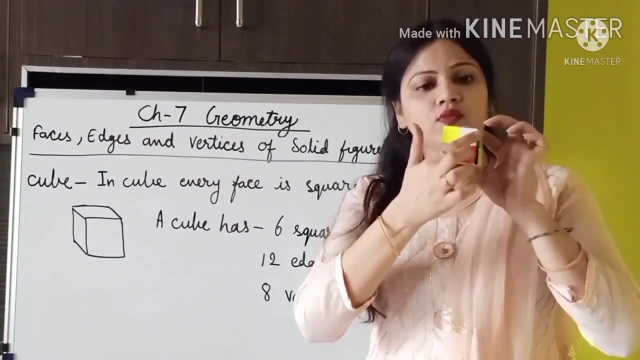 learn about the faces, edges and vertices of solid figures, Like here. I have drawn a cube shape, Cube shape. This is the cube shape. In the cube shape, every face is square. You can see, this one is also square. This one is also square. 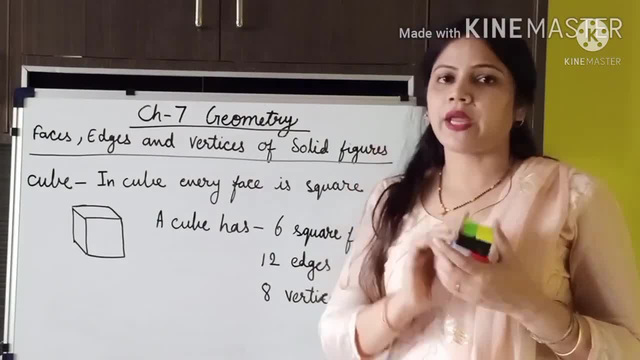 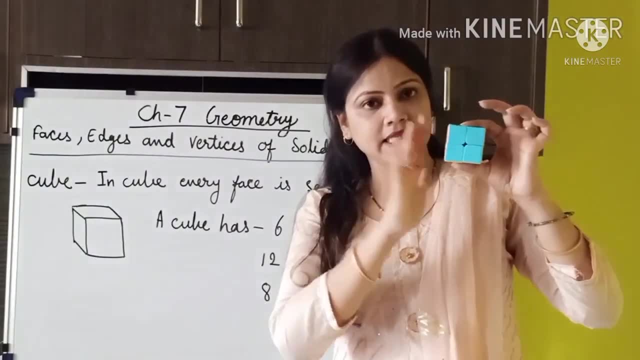 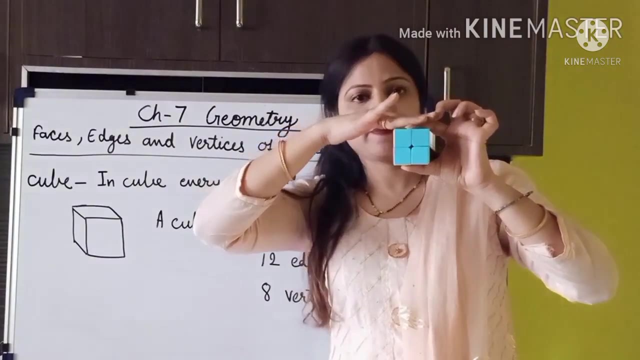 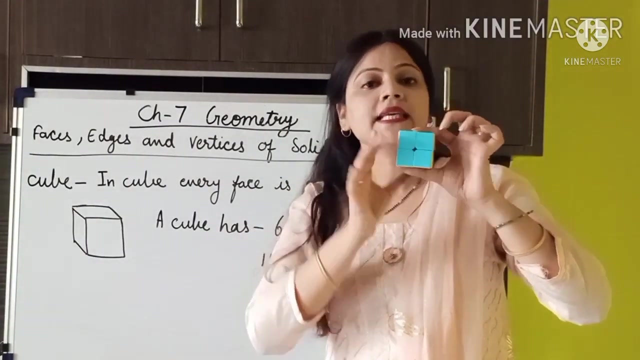 Similarly like that all the faces are square in shape. Okay, Now it has six square, flat faces, Six faces. It has six faces: One, two, three, four, Okay Five and six, Okay, Four sides, and one in the bottom and one in the top. You can see these are the six faces. 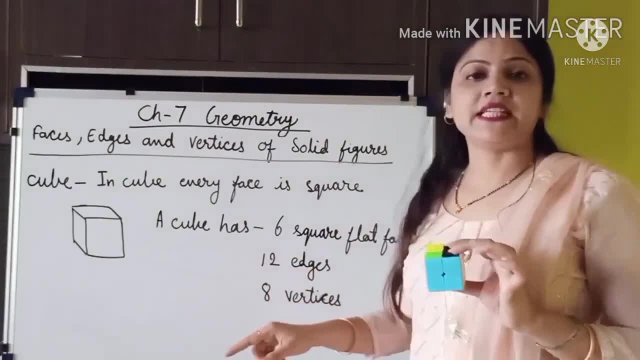 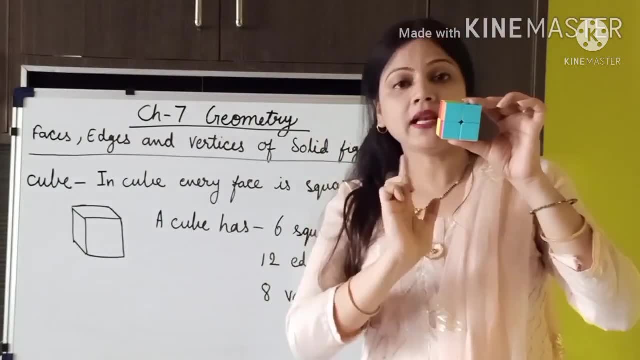 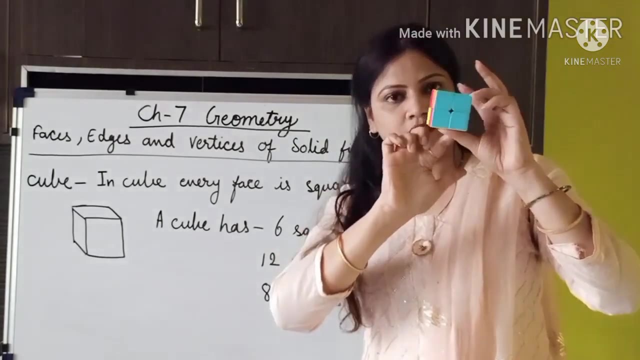 of this cube. Now it has twelve edges. Ages means side, This is called the edges. So this cube has twelve edges. How? One, two, One, two, three, four, Four, then five, six, seven, eight, nine, ten, Okay, Five, six, seven, eight, nine, ten, Okay, Five, six, seven. 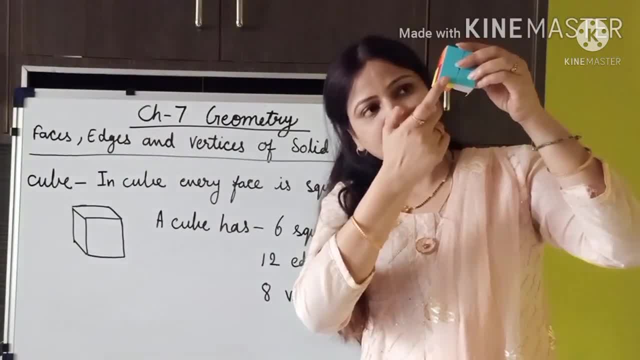 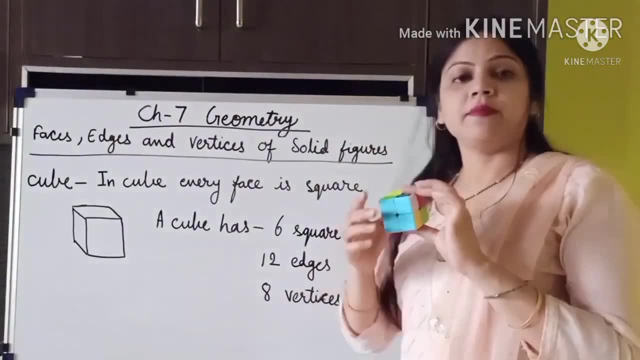 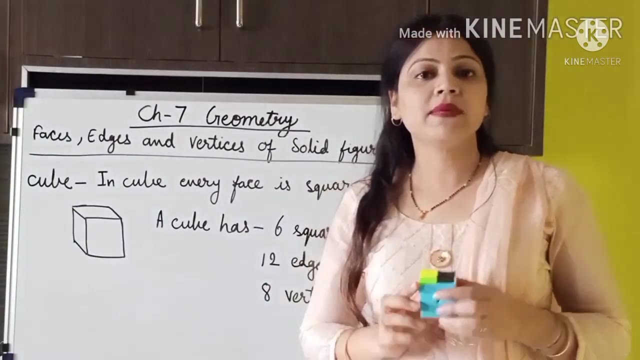 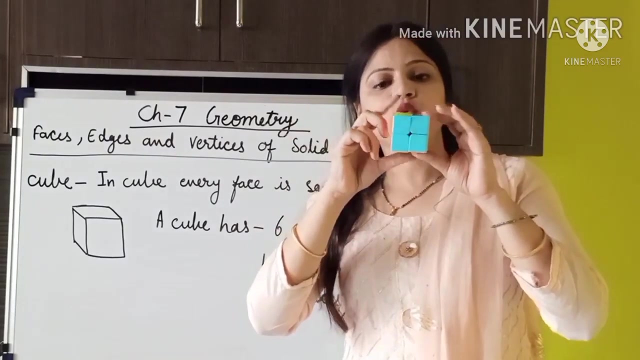 eight, And after that nine, ten, eleven, twelve. So a cube has twelve edges, Means twelve sides. Okay, After that a cube has eight vertices. Vertices means corner. This is called vertices, The corner. Okay, So it has eight vertices: One, two, three, four. 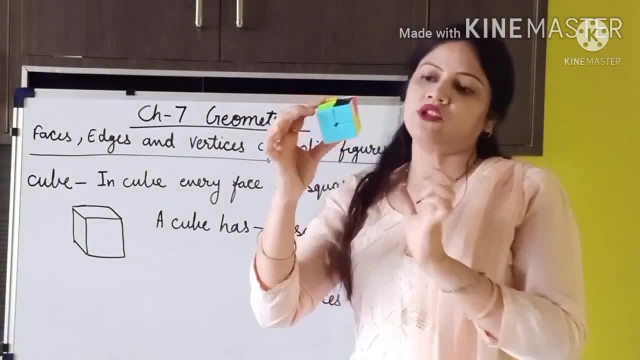 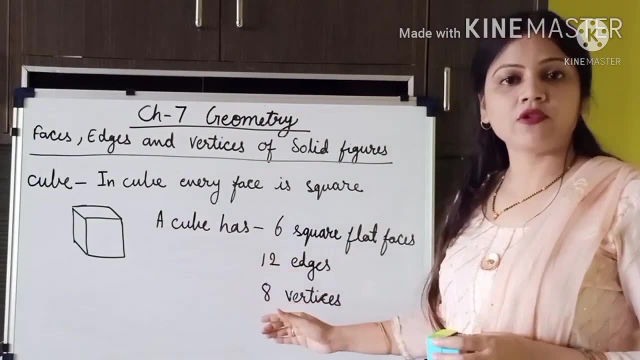 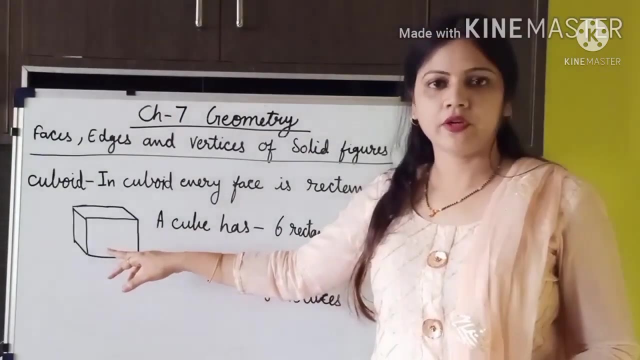 Five, six, seven, eight Understood. So this is the description of cube. You have to write these things. So just pause this video and write these things in your maths copy. Now, here I have drawn a cuboid. Okay, Cuboid. it is similar like cube, but rectangle in shape. 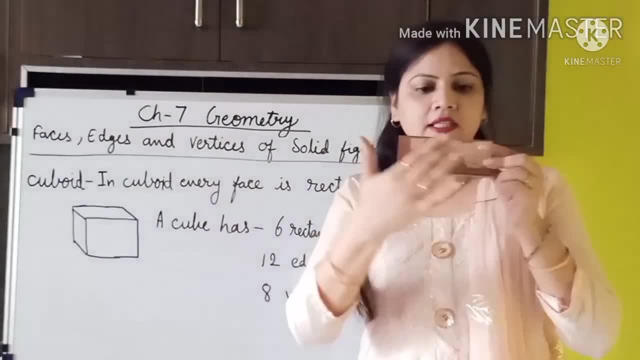 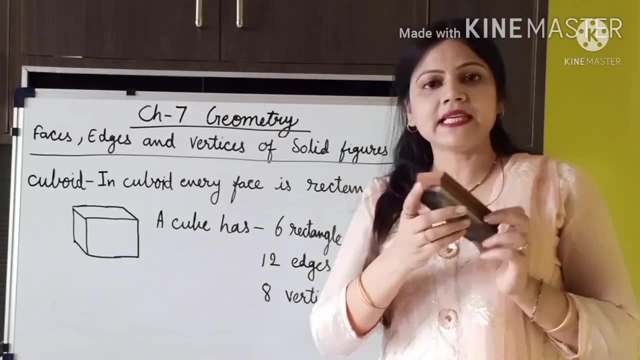 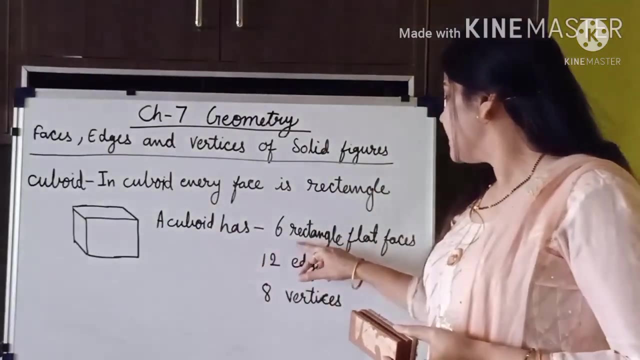 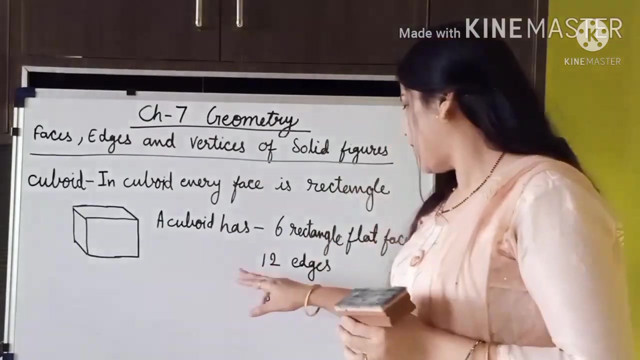 Okay, In cuboid, every face is rectangle. You can see, this one is rectangle, this one is rectangle. Okay, So every face is rectangle. This is also rectangle, Okay. A cuboid has six rectangle flat faces. These are the six rectangle flat faces, After that twelve edges. 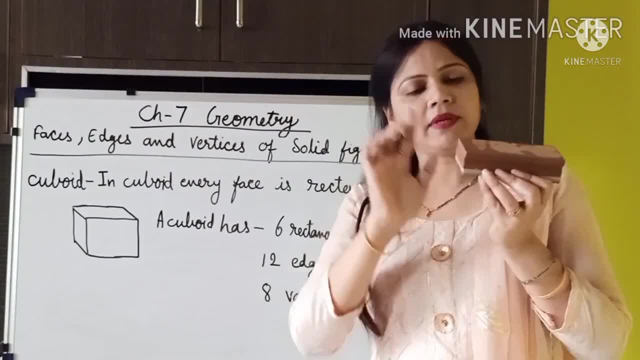 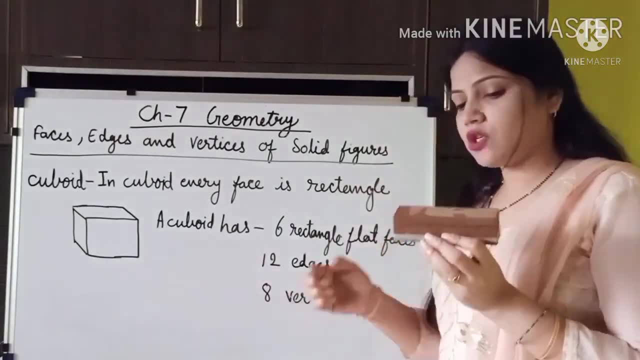 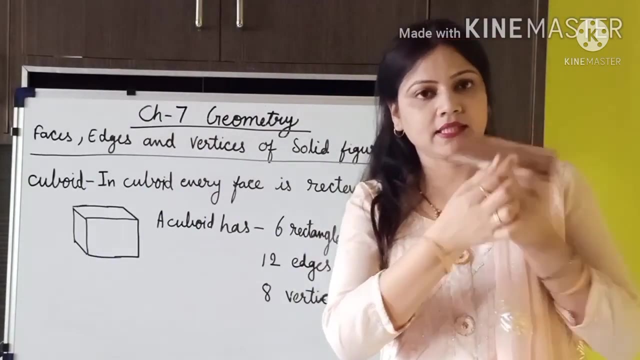 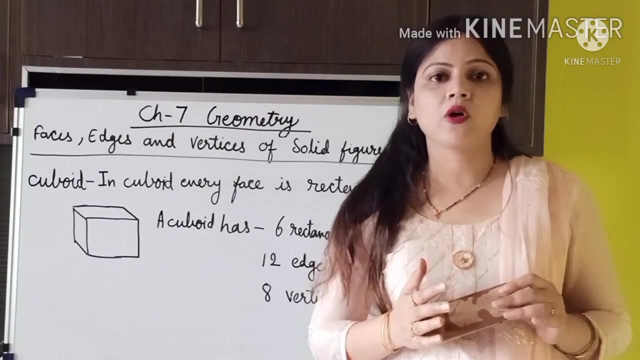 Ages means sides. It also have similarly like that cube. It also have twelve edges And eight vertices. Vertices means this corner, Okay. This cuboid have eight vertices, Okay. Some examples of cuboid are duster, tiffin box, pencil box, bricks. These are the examples. 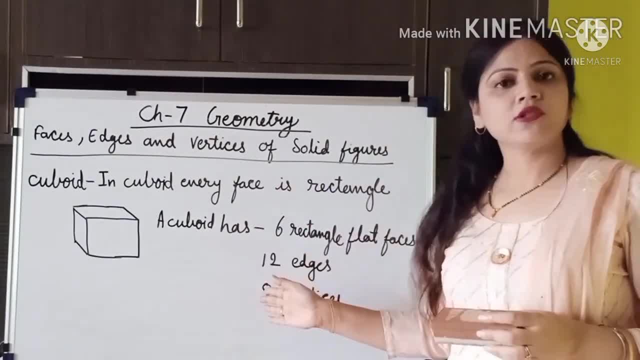 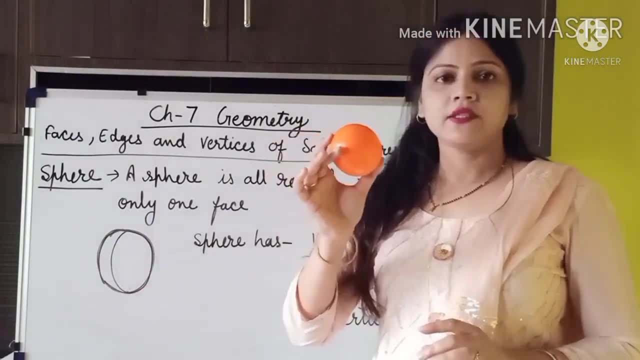 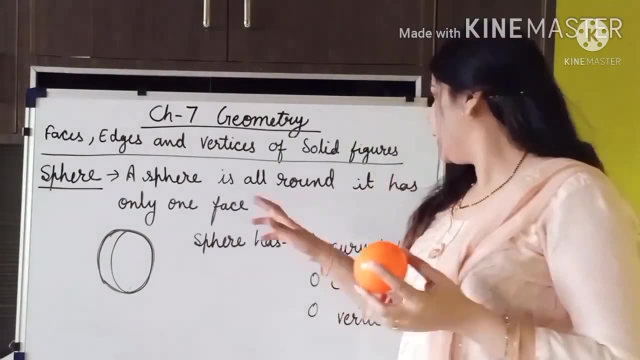 of cuboid. So just pause this video and write these things also in your maths copy. The third type of solid shapes are sphere. Like this You can see this is a sphere. Like this You can see a sphere is all round From wherever you will see this. this is round, Okay It. 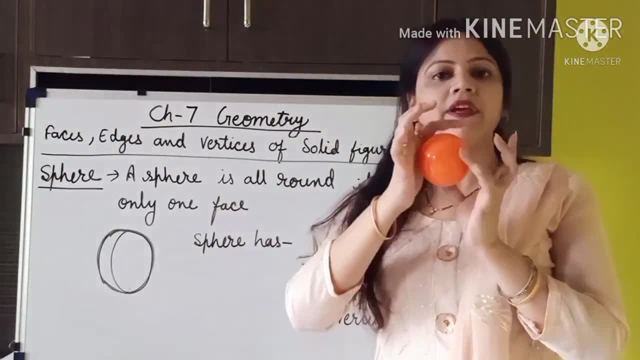 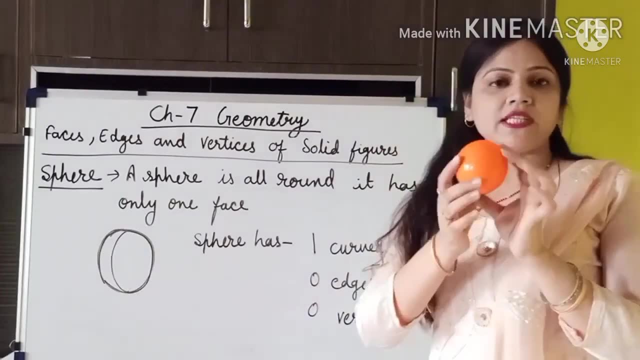 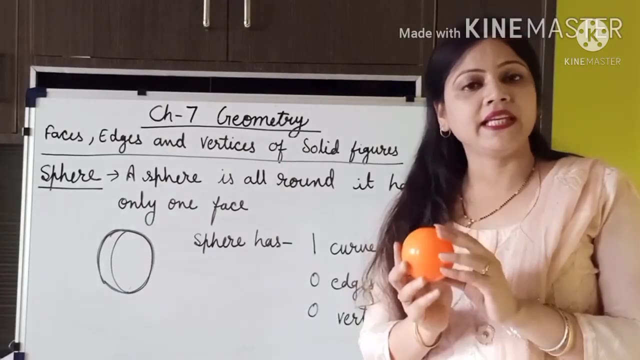 has only one face. It has only one face, that is, curved face. Okay, Now, a sphere has one curved face, Zero edges, As you can see. there are not any sides And zero vertices. It also don't have any corners. It has only one curved face. Okay, So you can see, this is a sphere. 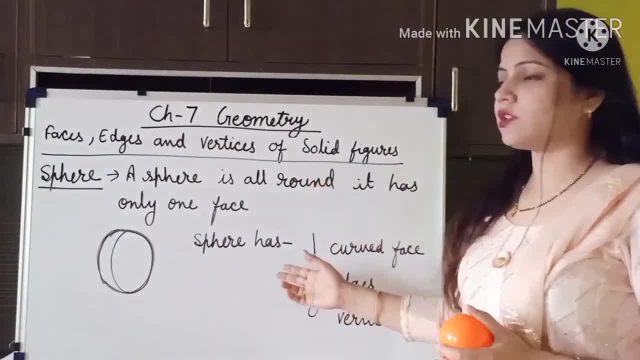 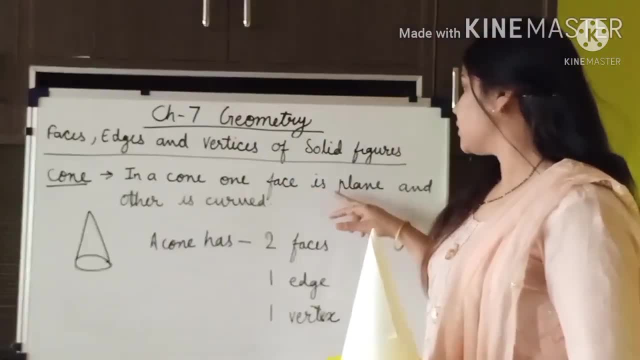 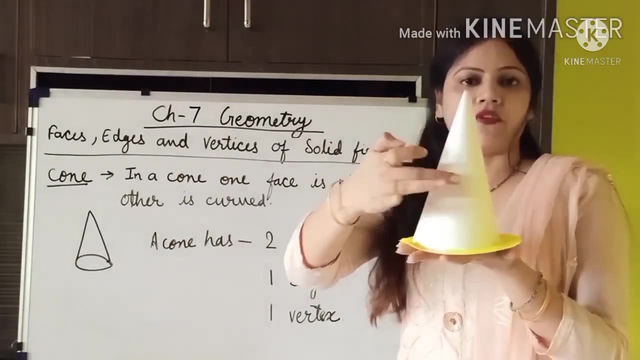 It has only one curved face, Okay. So just pause this also and write this in your maths copy. Now. the fourth type of solid shape is cone. It has one plain face and one curved face. As you can see, this is a cone. This is the curved face, Okay. Wherever you will see this, 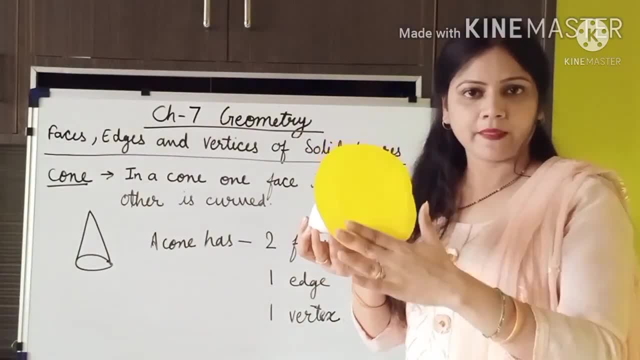 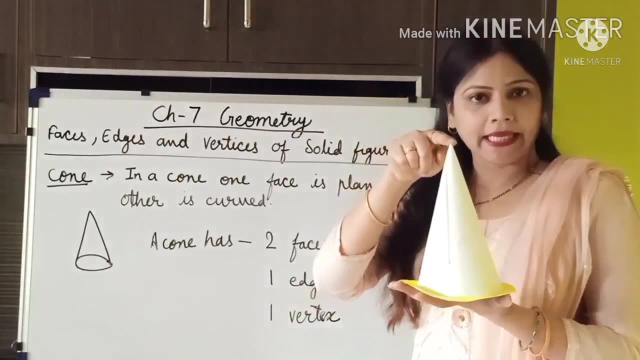 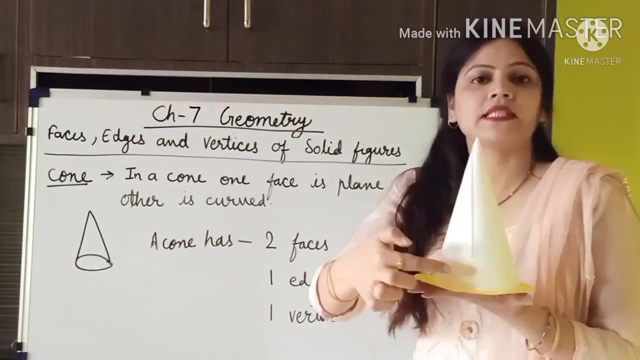 is curved only And this is plain face. Okay, So this one plain face and one curved face. It has one vertex- Corner is called vertex. Okay, So it has one vertex and one edge, The sides one edge. Okay, So just pause this and write these things in your maths copy Now. 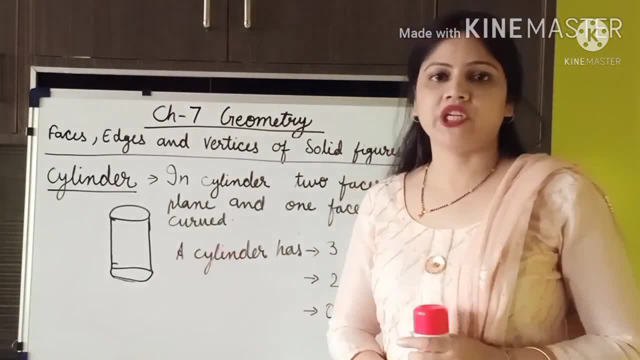 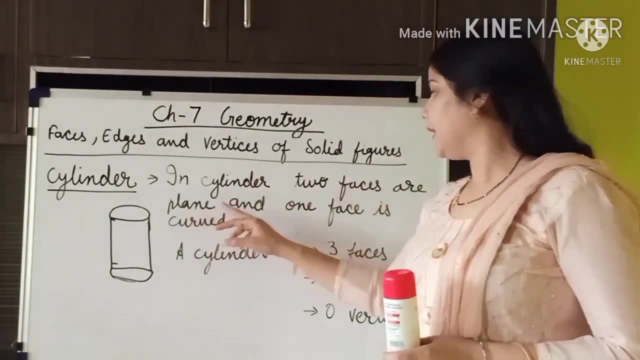 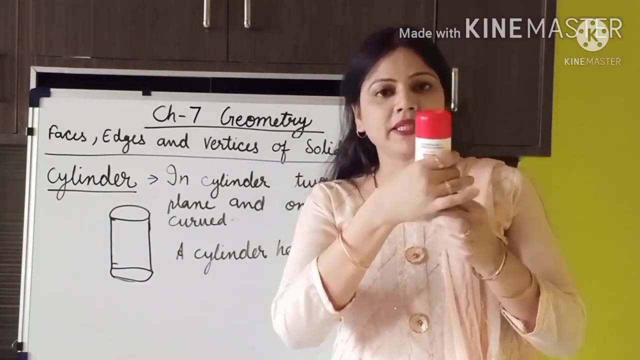 we will look for the last solid shape, That is, cylinder shape. Okay, It looks like this. Okay, In cylinder, two faces are plain and one face is curved. As you can see, the top and bottom face is plain, while the middle, this area, is curved face. Now a cylinder. 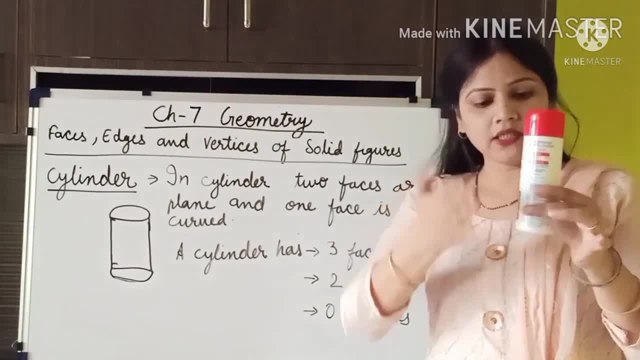 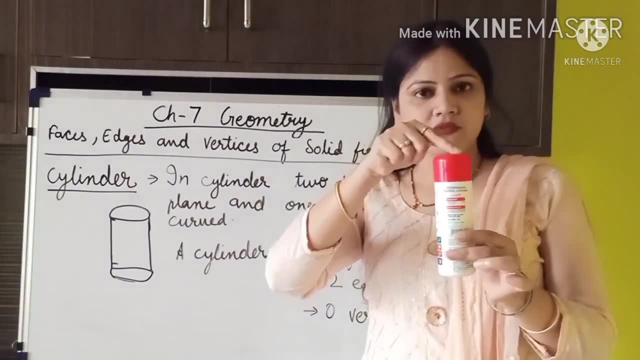 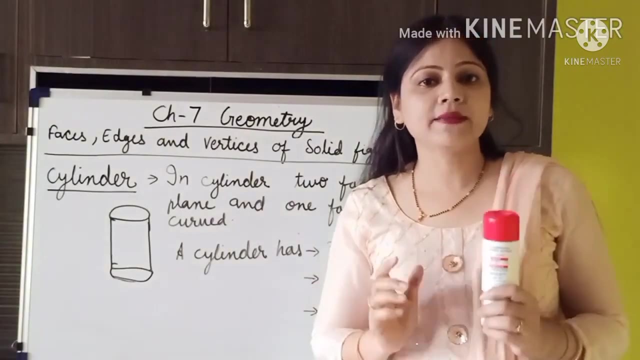 has three faces, As you can see: two faces, One, two and this one is three. Three faces, Two edges. Two edges are there, First one, this edge, and second one, this edge. Zero vertices. Vertices means Vertex means the corner. You can see any corner here. No, This cylinder. 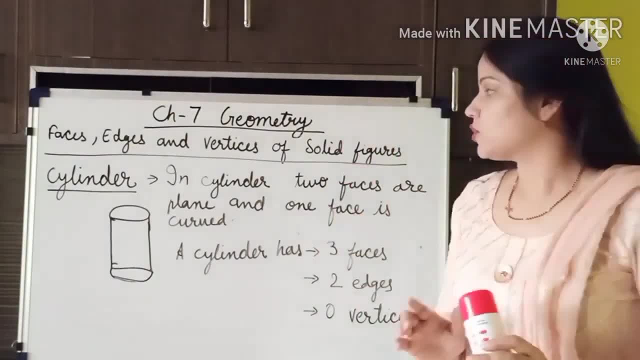 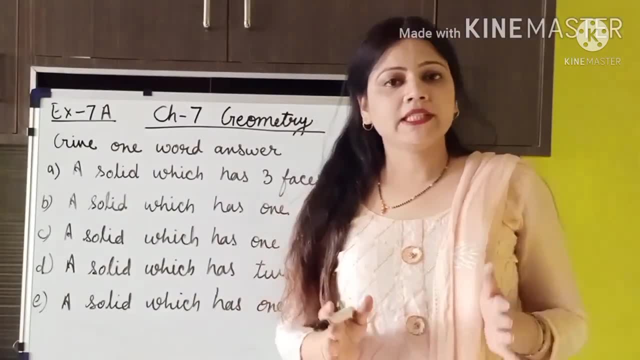 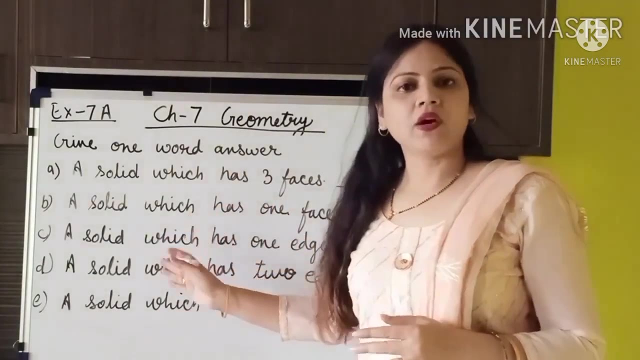 shape has zero vertex. So just pause this also and write these things also in your maths copy, Okay, So, according to the shapes- solid shapes- that I already have taught you here, I have given some questions. Okay, So we will just try to find out the answer of these questions. 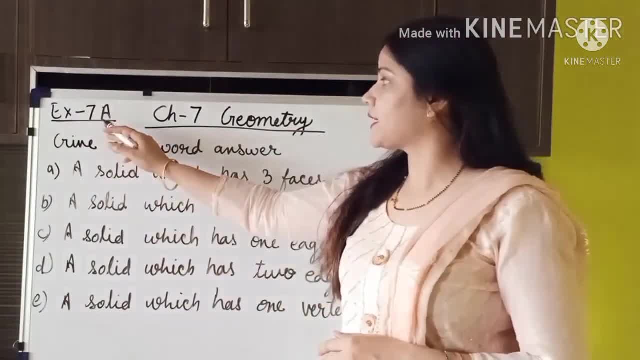 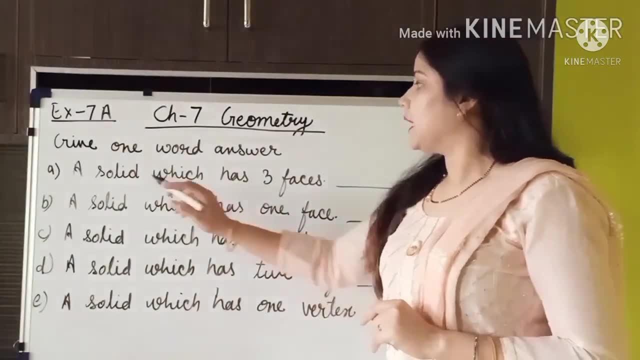 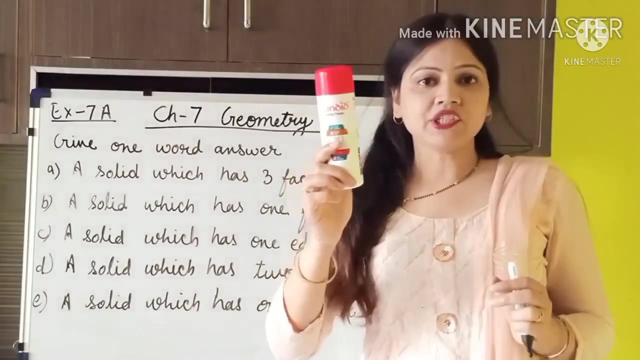 This is of. these questions are of exercise seven, eight. Okay, What we have to do? Give one word answer. We have to write only one word answer here. A solid shape has zero vertex, A solid which has three faces. So if you have remembered that cylinder shape has three.